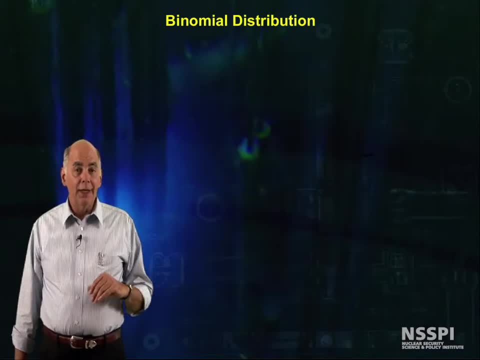 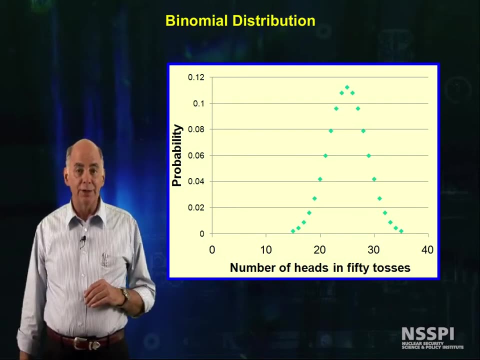 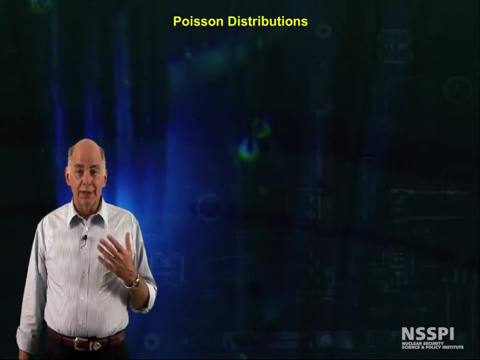 average or the expected value does it Again courtesy of Excel, here is a graph of the probability of getting a particular number of heads and 50 tosses of a fair coin, If the number of observations is large and the probability of success for any. 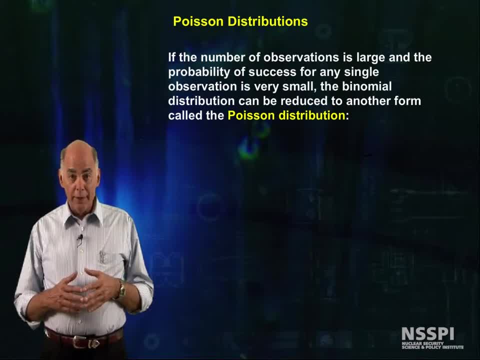 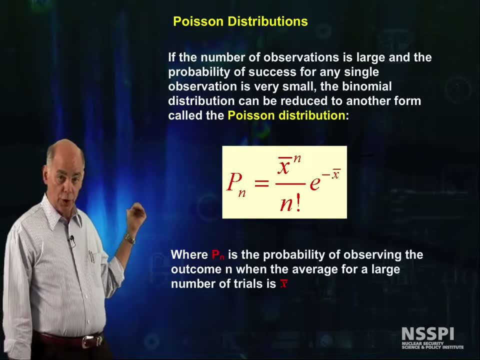 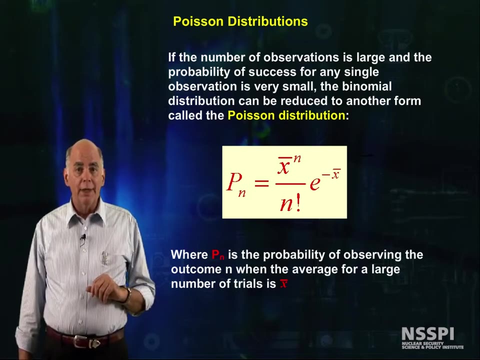 single observation is very small. the binomial distribution can be reduced to another form, called the Poisson distribution shown here, Where P sub N is the probability of observing the outcome, little n, when the average for a large number of trials is x bar. 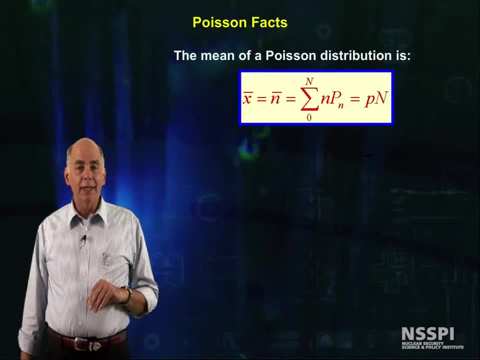 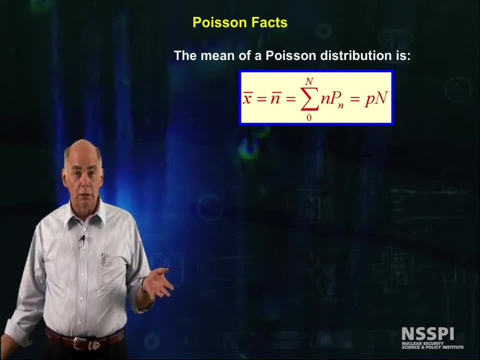 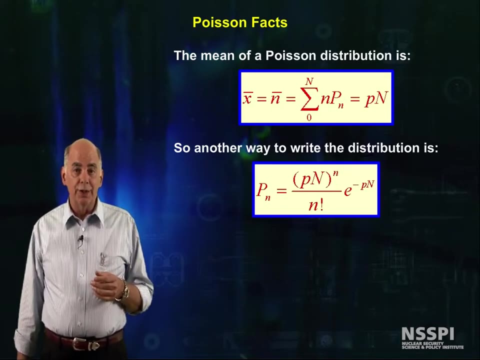 It. It can be shown- but let's don't do it here- that the mean x bar of the Poisson distribution is just the probability per trial times, the number of trials, or big P times big N. So another way we can write the distribution is instead of writing it in terms of x bar. 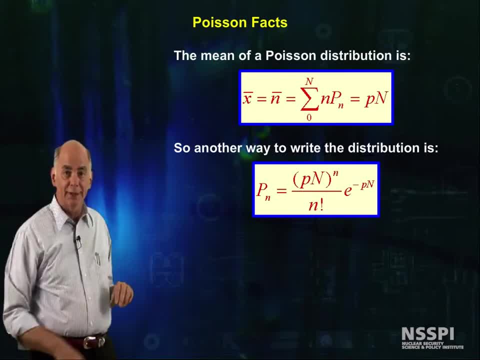 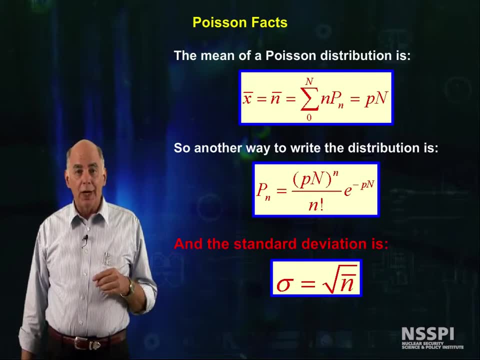 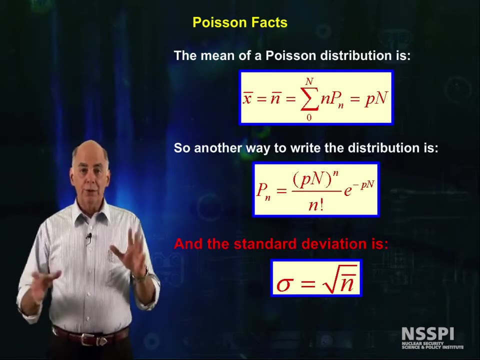 we can write it in terms of P- N. It makes some people happier to write it this way. The important fact for us nuclear types is that the standard deviation of a Poisson is just the square root of x bar the expected value. So let's regroup here and look at: 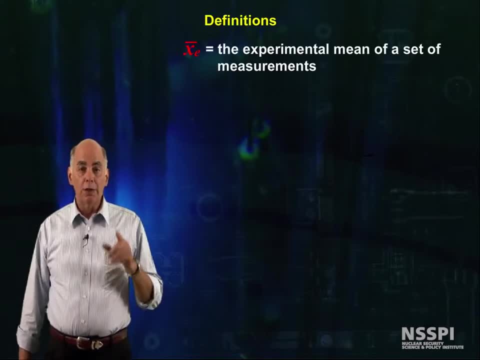 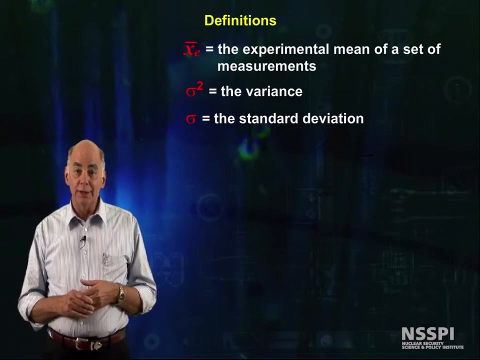 some definitions. Let's define x bar, sub E- oh wow- as the experimental mean of a set of measurements. Sigma square is the symbol that statisticians use for the variance. The variance is just the square root of x bar. We expect the distribution for a set of measurements to be well approximated by a Gaussian. Huh, 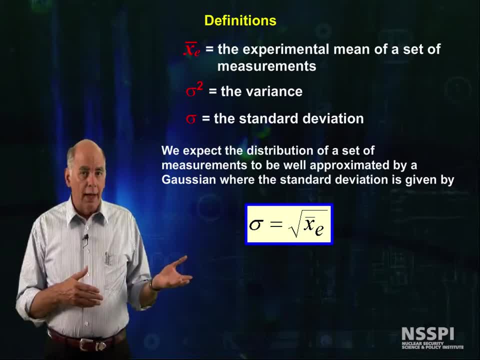 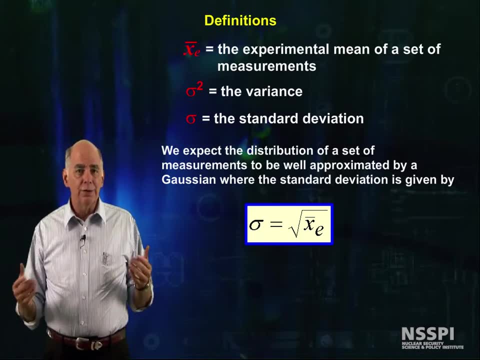 Why a Gaussian and not a Poisson? And the standard deviation is given by the square root of x, bar, sub, E. Huh, On the surface this makes no sense at all. Poissons are for discrete values. integer counts the square root of x, bar, sub, E. Huh, On the surface this makes no sense at all. Poissons are for discrete values. integer counts the. 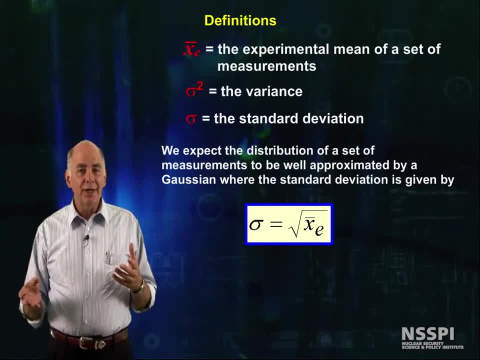 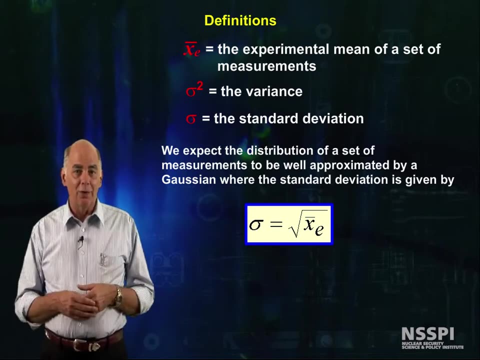 number of times you flip heads. Gaussians are set up for real numbers. Last I checked, counts are most definitely not a real number. right, It's really hard to get 14.27 counts, But it turns out, and I'll show you in just a second. this works very well. So for radiation,